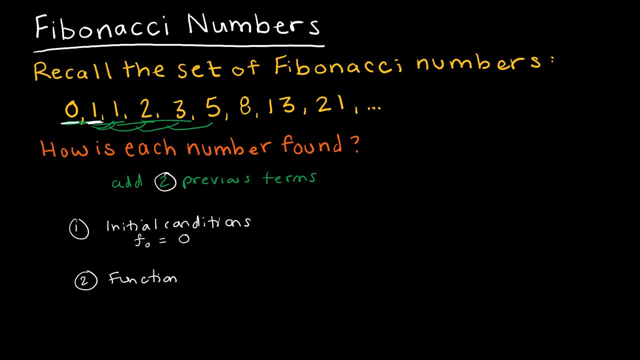 象. I said the first term is 0.. It starts with the second word first, and then it starts with the, And then our first value after that is one. so we start with the 0, which is the starting point, And then the function has to define how to find the next term in the sequence. So f of n is found by taking 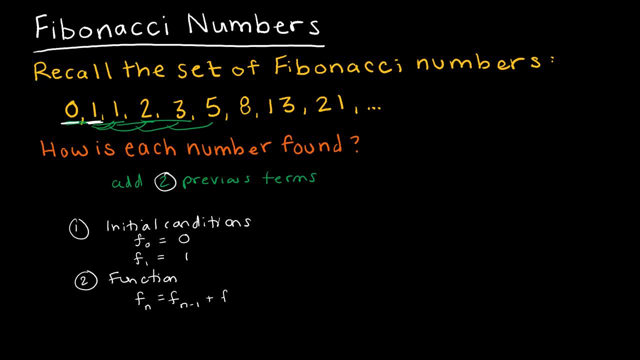 the term right before that and the term right before that, And we should also include that n has to be greater than or equal to 2.. And I'm including greater than or equal to 2 because we've already defined 0 and we've already defined 1.. So this is how we defined it previously. 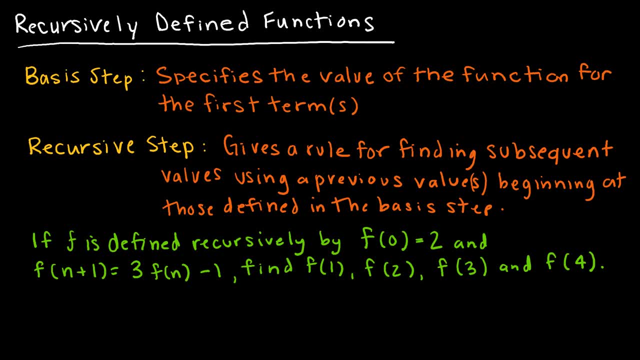 So now let's look at what I have written here. A recursively defined function has two parts: a basis step and a recursive step. And you might be thinking: well, that sounds pretty familiar to what we were just doing with mathematical induction, where we had a basis step and an 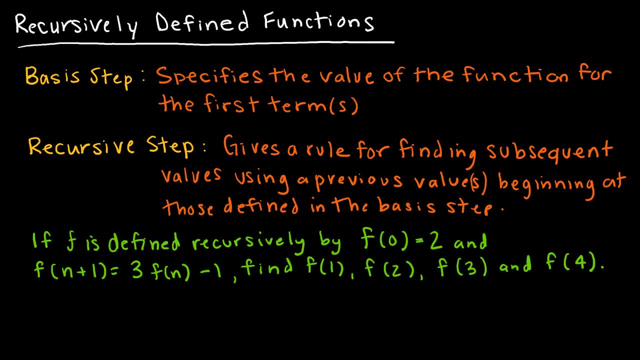 inductive step, And you're absolutely right, This is going to flow right into proofs with recursive definitions. Now, the basis step is the same as the initial conditions that we talked about before. It specifies the value of the function for the first term or terms. 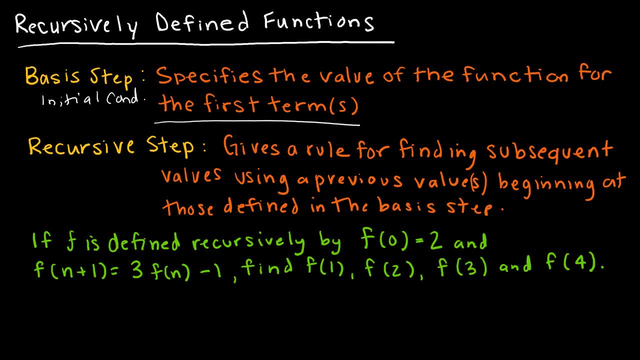 So that's what those initial conditions were before and that's what they are again. The recursive step gives us a rule for finding subsequent values using previous values. So this is the function. So for instance I have: if f is defined recursively by f of 0 equals 2,. 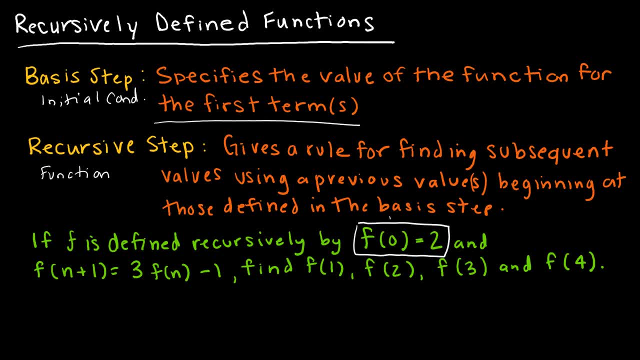 that would be my initial condition or my basis step, And f of n plus 2 is my basis step. So that's what those initial conditions were before and that's what they are again. 1,, meaning the next term in the sequence, says: take the term f of n, multiply it by 3, and subtract 1.. 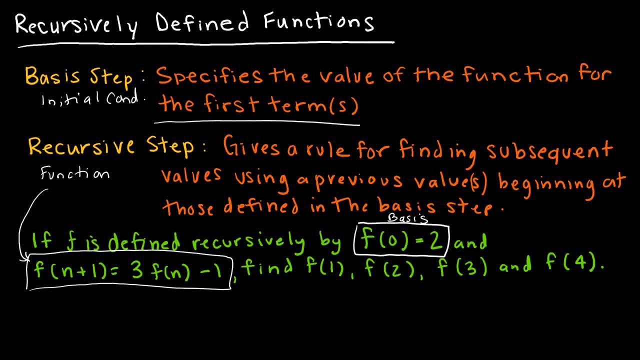 So that would be the function. So I want you to notice some difference here. just so we can point out what may already be obvious to you. This one is defined as f of n plus 1.. I could also say this is to find f of n. I'm going to take 3 times f of n minus 1, minus 1.. So again, it's just saying: 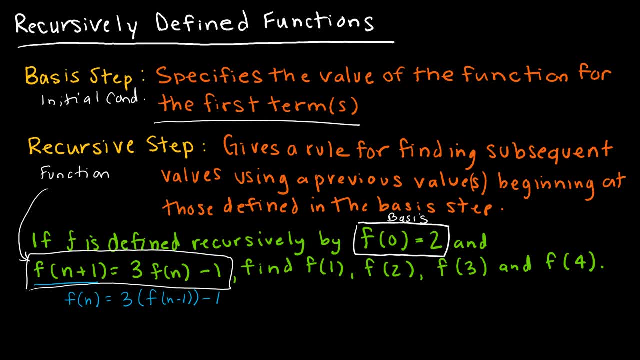 take the term before that, multiply it by 3, and subtract 1.. So either way that you write that, that could be just fine. So let's start with f of 1.. To find f of 1, it's saying: take 3 times. 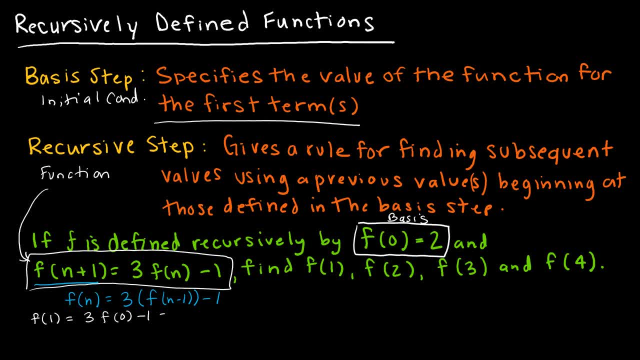 f of 0, minus 1.. Well, f of 0, we wouldn't know unless we had our basis, our initial condition that f of 0 was 2.. So I'm going to take 3 times 2 minus 1,, which is 6 minus 1, or 5.. And then to find f of 2,. 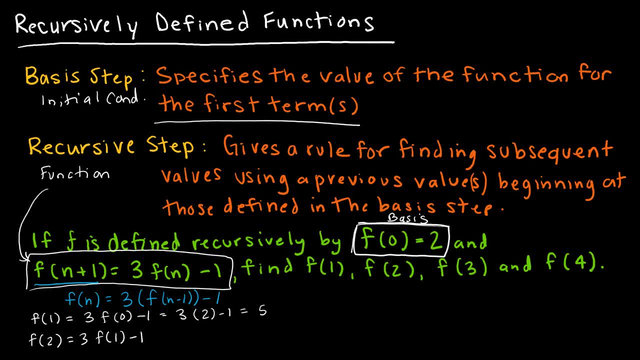 it says to take 3 times f of 1, minus 1.. So 3 times 5 minus 1 is 14.. And then to find f of 3, because we're asked to find 1,, 2,, 3, and 4.. So f of 3,. 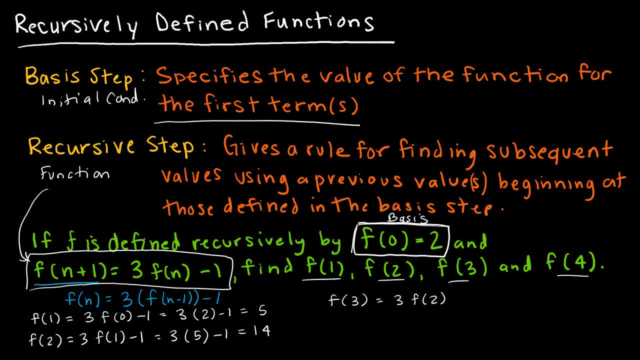 would be 3 times f of 2, minus 1,, which is 3 times 14, minus 1,, which is 41.. And then f of 4, which is 3, f of 3's minus 1, which is 3 times 41, minus 1,, which is 122. 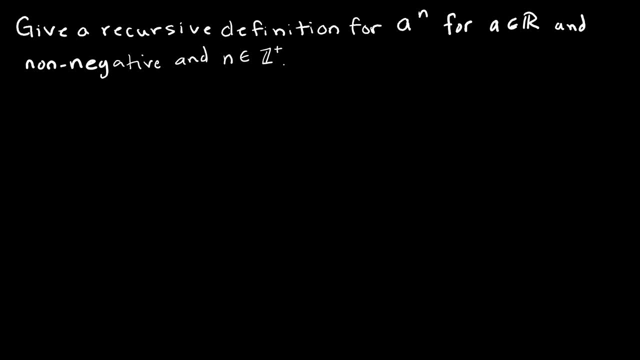 Let's see if we can find a recursive definition for the function a to the n, where a is some real number that's non-negative, and n is some positive integer. So again, whenever you're trying to find a recursive definition, there are two. 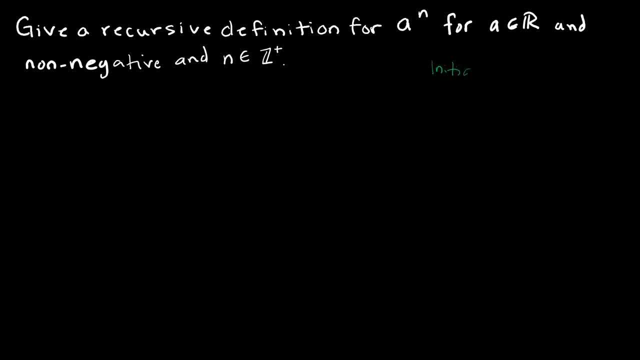 parts. There's the initial condition or conditions, and then there's the recursive function, And you could actually say that there's three parts, because you need to make sure that when you define the recursive function you have to define for what values of n. So that's sort of a implied third part. So there's two main parts. 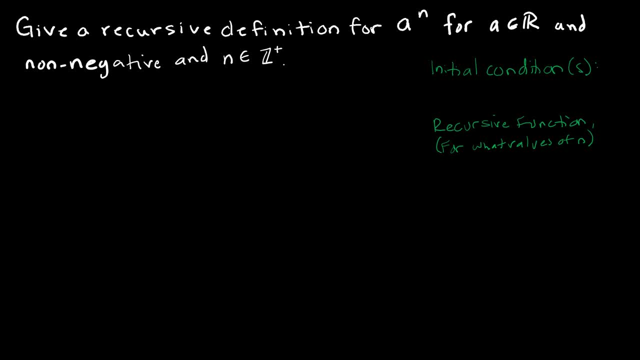 So let's take a look. If I have a to the n, then a to the 0, and anything to the 0 is 1.. a to the first is just a. a squared is a times a. a cubed is a squared times a. a to the fourth would be a cubed times a, And we can see. 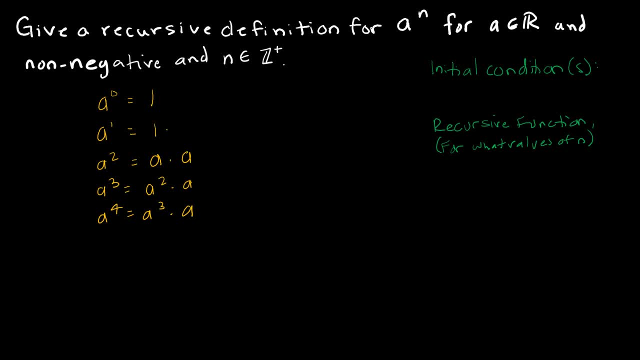 the way that I'm writing this, I can see that there's some sort of pattern here, And the pattern appears to be that I'm going to multiply, so i'll multiply by a, by whatever I had in this step before. so again, that's the recursive. part of this is that I'm taking 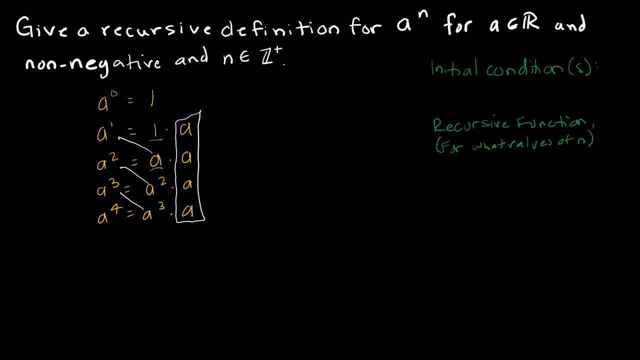 something that I had before and that I'm doing something to it to find the next value. So this made it very easy to come up with the two parts. My initial condition is that a to the zero power is 1.. And then, if I want to find a to the n. 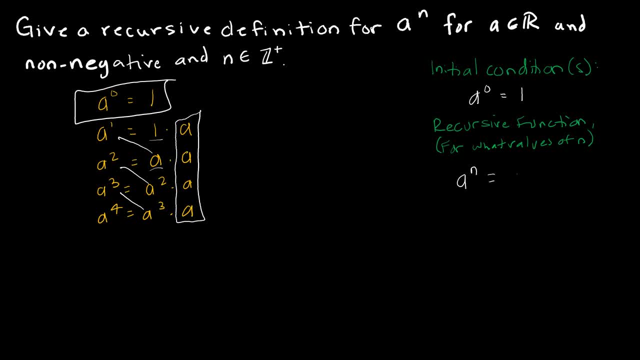 nth power. all I have to do is take a to the n minus 1th power, so whatever power I had before, and multiply it by a. Now, for what values of n is that valid for? That means for n greater than or. 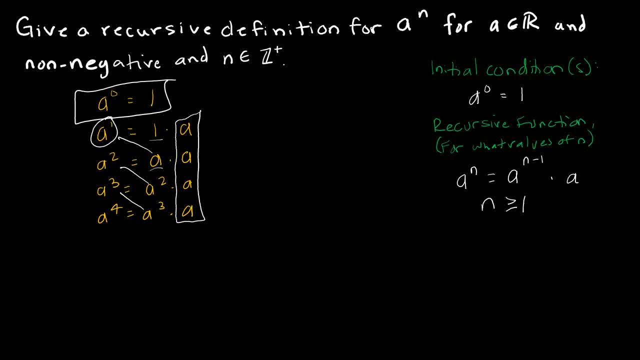 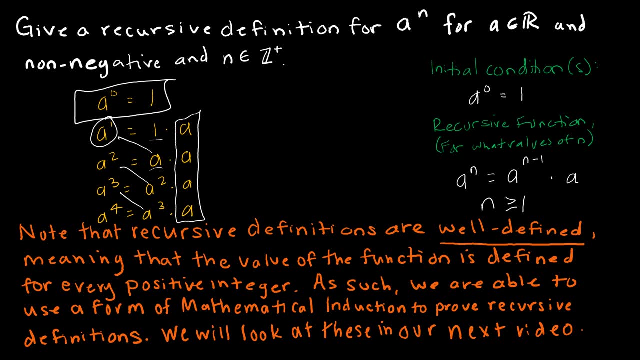 equal to 1, because I'm starting that recursive definition at 1.. Keep in mind that a recursive definition is considered well-defined, meaning that the value of the function is defined for every positive integer, and therefore, in a little bit we'll be able to use a form of mathematical 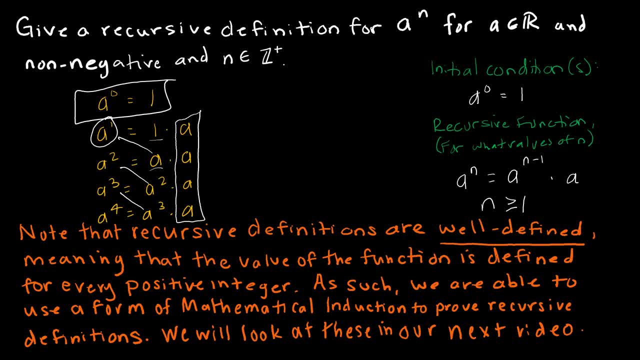 induction to prove recursive definitions are true. So right now we're just looking at this and saying, yep, this is true because I said so and of course I can always plug values back in to check. but we can actually do a form of mathematical proof to prove that the recursive 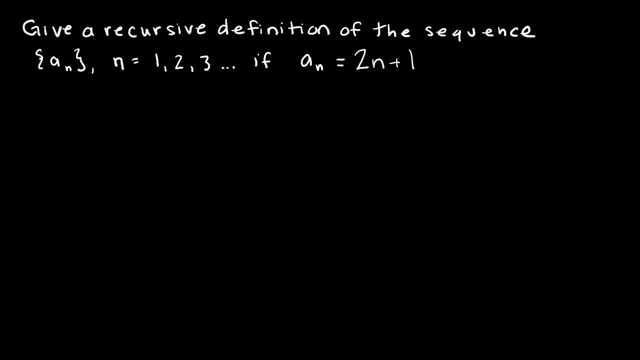 definition is true. Let's take a look at another question. We're trying to find a recursive definition of the sequence: a sub n where a sub n is 2n plus 1, and again I'm going to start it the same way. I'm going to find a sub 0, a sub 1, a sub 2,, a sub 3,, a sub 4, and see if, based on 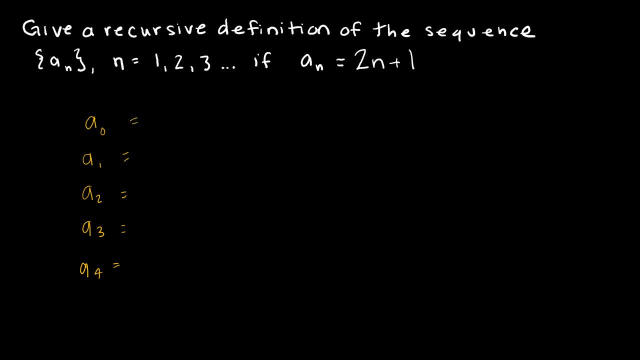 those values, I can find some sort of pattern. So a sub 0 is 2 times 0, and a sub 1 is 2 times 0, plus 1, or 0 plus 1,, which is 1,, and then a sub 1 is 2 times 1 plus 1,, which is 2 plus 1, or 3.. 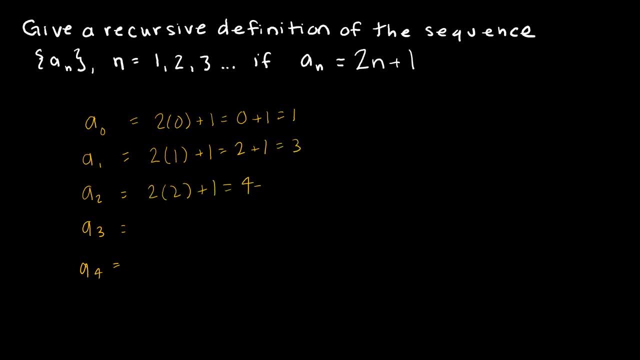 a sub 2 is 2 times 2 plus 1, or 4 plus 1,, which is 5.. a sub 3 is 2 times 3 plus 1, and we get the idea here: 6 plus 1,, which is 7, and then I can take 2 times 4 plus 1,. 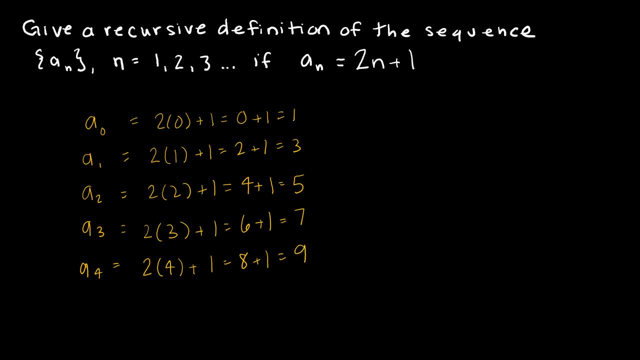 is 8 plus 1, which is 9.. So I have a very established pattern here. Comparing one value to the next, it appears that all I have to do to get from one to the next is add 2.. So again, 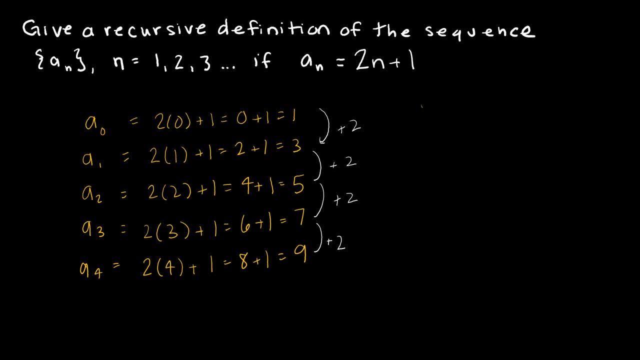 let's take a look at how we might write our definition. First, I'm going to write my initial condition, And my initial condition would be that a sub 0 has to be 1.. So I'm going to set that to be my initial condition, And then from there I know that all I have to do is write my recursive. 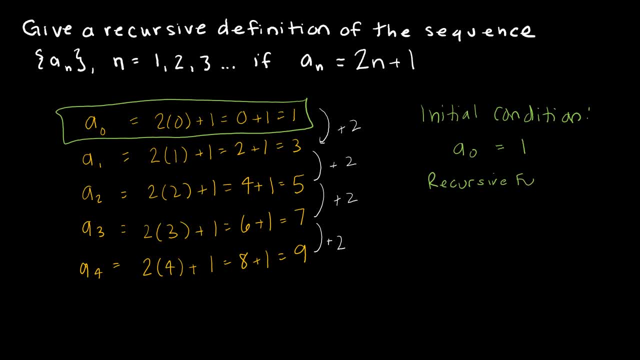 function which is going to define what a sub n is, And my recursive function here is that I would take whatever the value was before which is a sub n minus 1, and add 2.. And that's going to be for all n values greater than or: 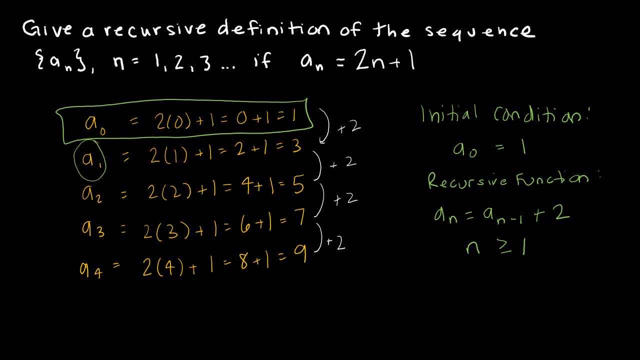 equal to 1, because a sub 1 is where I'm first going to be able to find the solution, using my initial value of 1 and adding 2.. And again, if you're ever unsure, you can always plug values back in to make sure. So a sub 1,, according to my new recursive definition, is a sub 0 plus 2.. 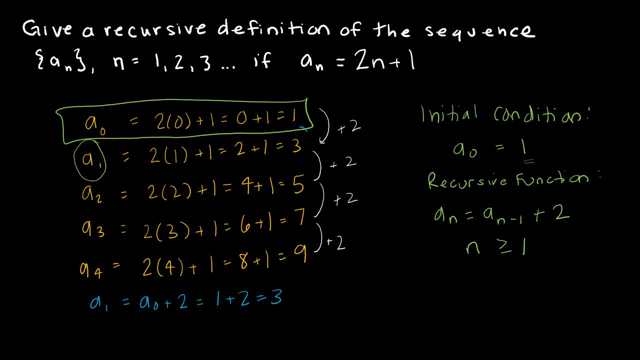 Which is 1 plus 2 or 3,, which matches up, And then a sub 2 is a sub 1 plus 2,, which is 3 plus 2,, which is 5,, which matches up. So you can always check it. But again, keep in mind, this is what 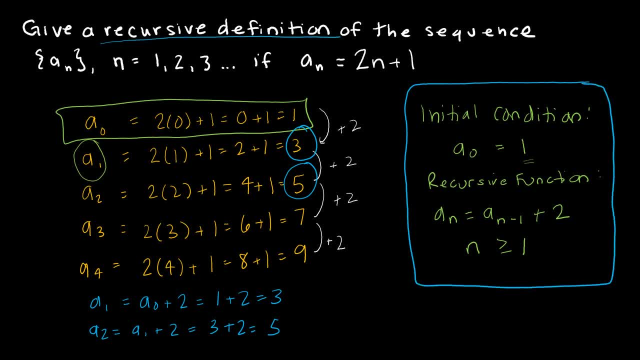 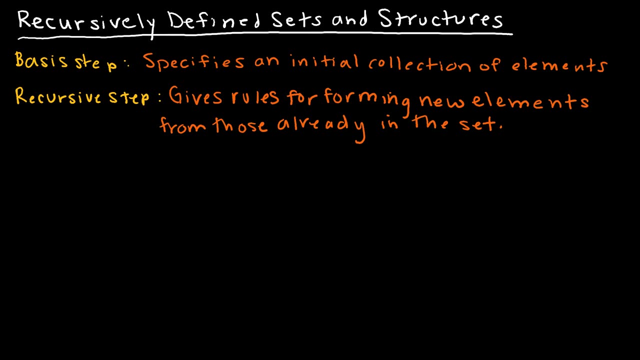 we're looking for. when we say find a recursive definition, We're saying: give that initial condition, give how to find the next value and then make sure you explain for what values of n that's valid for. It's important to understand that to this point, all we have done is define functions recursively. 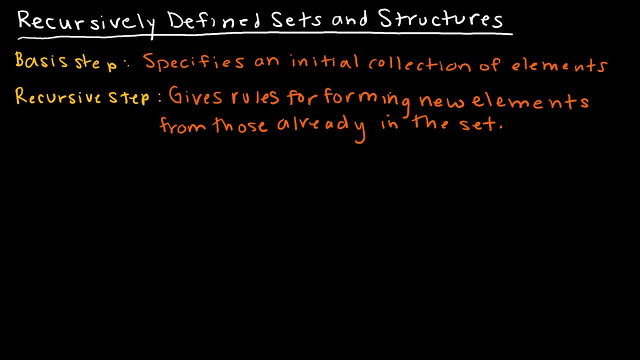 but we can also define a set or a structure recursively. So the next several examples will be sets or structures. So, for instance, again the basis step- and I'm going to focus specifically on a set. this time the basis step will specify an initial collection of elements. 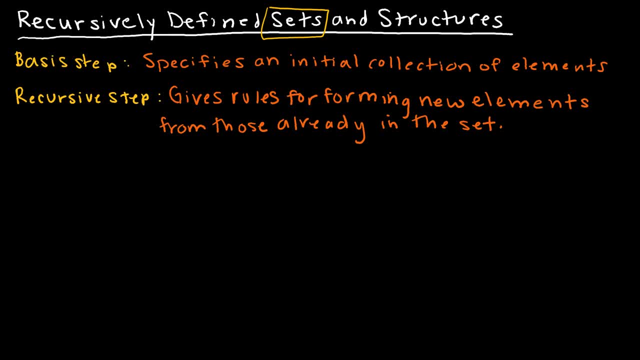 And the recursive step will give a rule for how I'm going to find the next element based on the previous elements. So let's do an example with, say, the natural numbers, And, if you'll recall, previously the natural numbers were just the counting numbers. 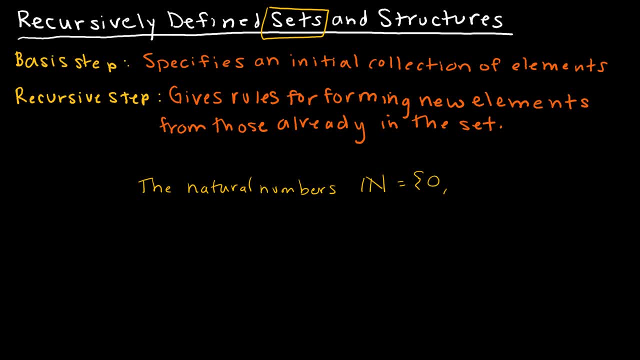 which is 0,, I'm sorry, not 0. We don't start at 0 when we count 1,, 2,, 3, and so on. So if our were to define the natural numbers recursively, I would again have a basis step And my basis step. 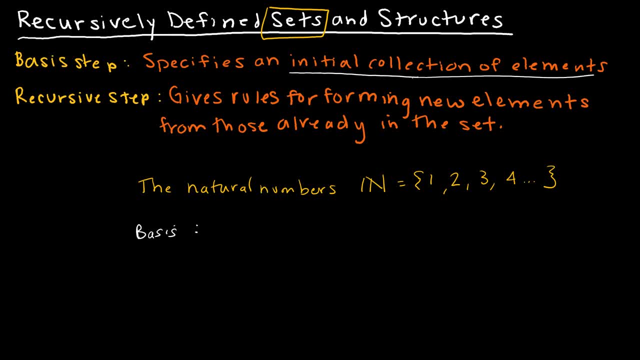 would specify an initial collection of elements. So in this case, I'm just going to say what the initial value is, that 1 is a natural number. Now the recursive step tells me how to get to the next number based on the initial collection of elements. So in this case, I'm just going to say: 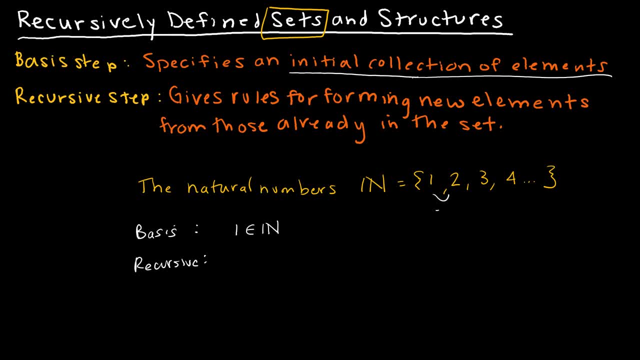 what is n, which is 1, and plus 1,, which is the first essential value of the set. So the next item that we're going to be discussing is tab 4.. The first essential value of n is the value for any element, soظ 16.. The next item is the entry value, which is n. so we now add jap. 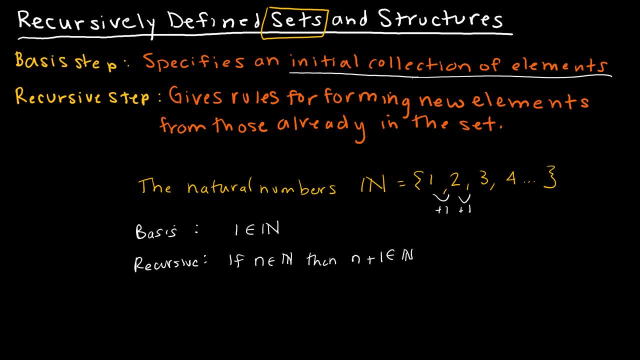 which is n and記 2.. Enjoy that of definition. So the basis says: start at 1, and then the recursive step says: if n is a natural number, so 1 is a natural number, then I can add 1, and that will be a natural number. And then if 2, 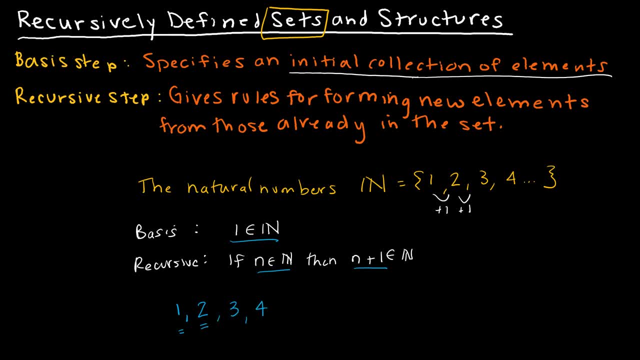 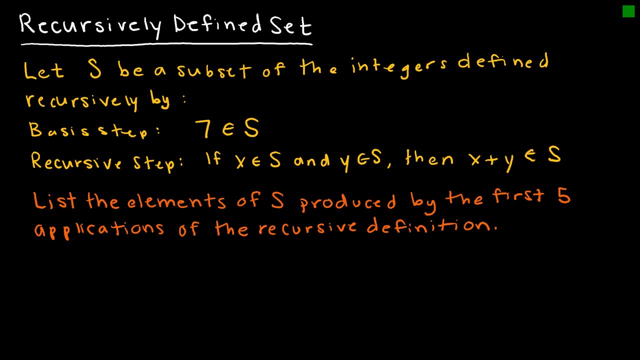 is a natural number. I can add 1, and that will be a natural number. And then I can add 1 and add 1, and we can see that we've defined it correctly. So let's look at another recursively defined set. 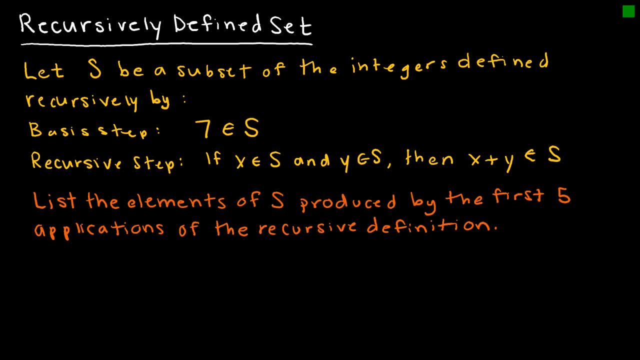 and that set says S is a subset of the integers defined recursively by the basis step, that 7 is an element of S and the recursive step that if x is an element of S and y is an element of S, then their sum is also an element of S. So if we wanted to use that to list the elements of S, 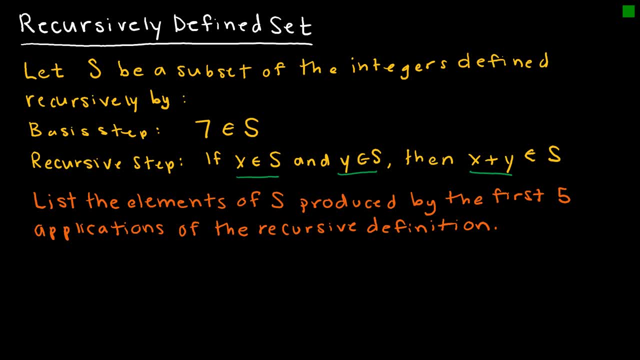 produced by the first five applications of the definition. the first value would be 7, because the first-fifth-fifth is an element of S. So if we wanted to control the set of N Number value comes from the basis step. So I've applied it once, Applying it a second. 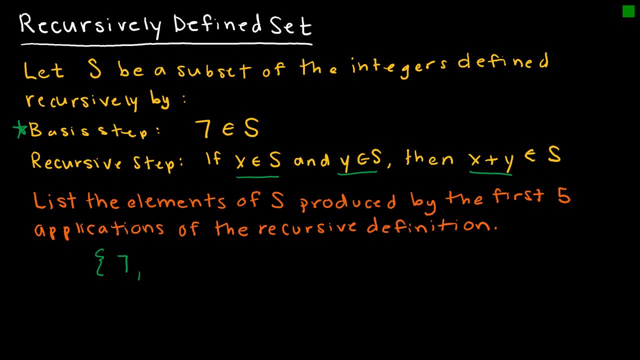 time gives me the first recursive step, which is, if X is an S and Y is an S, then X plus Y is an S, and so essentially that's saying 7 is an S and also 7 is an S, and so the sum of 7 and 7, which is 14, is an S. So that's really step 2, because 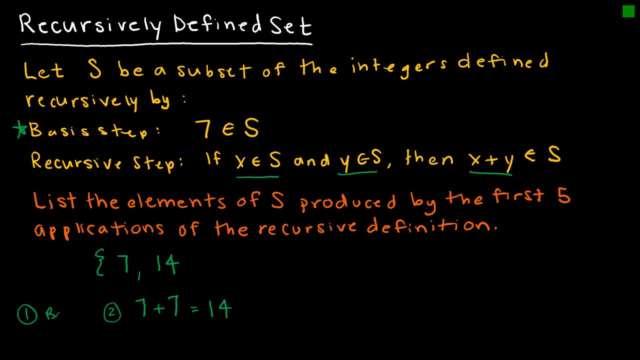 step 1 was the basis step that said 7 is in there. then step 3 says if X is an S and Y is an S, then the sum of those is an S, which is 21, and you can see this process. if I'm doing it 5 times, I would then take 7 plus 21 and that's 28 only. 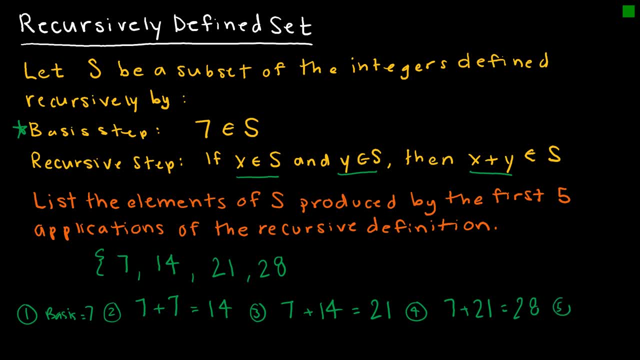 and, and then I'm talking about one more two. So this whole thing of whether it's an S or a, then 28 plus 7, and that is 35. Now you might be asking then: well, why wouldn't I add 14 and 35? 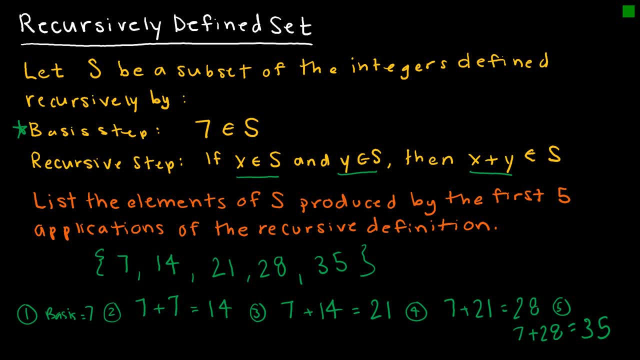 together. Why couldn't that be a step? And it certainly could be a step. I just wanted to get the first five applications, which is essentially that I'm adding 7 each time, And notice, if I took 14 plus 35,, that number, which is 49, would in fact be what I would get if I took 42,, which is 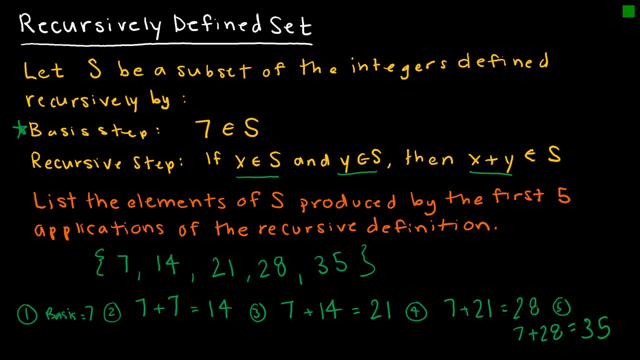 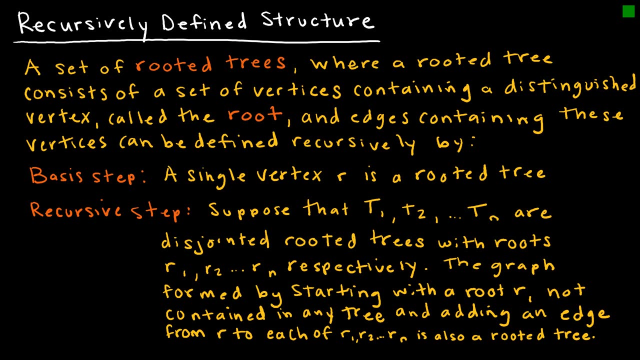 what the next value would be plus 7.. So I can add two other elements of the set together and that sum would also be in the set. I just wanted the first five. So I wanted to give you an example of a recursively defined structure rather than just a set, and I chose a rooted tree because we're 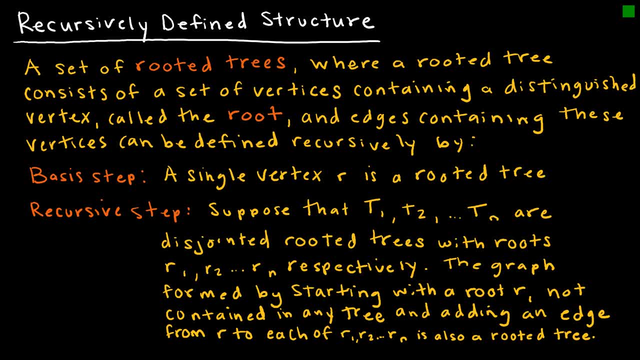 going to study rooted trees in an upcoming video, So I'm going to go ahead and do that, And so I wanted to give you a good introduction. So this says a set of rooted trees, where a rooted tree consists of a set of vertices containing a distinguished vertex called the root and edges. 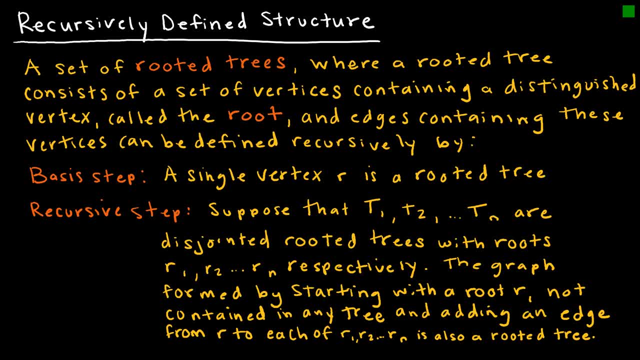 containing these vertices can be defined recursively by the basis step. that says: I have a single vertex. So let's say here's my single vertex R, that is a rooted tree. The recursive step says: suppose that you have tree 1. Tree 2. Tree 3, etc. All disjointed rooted trees. Disjointed means they're not connected to one. 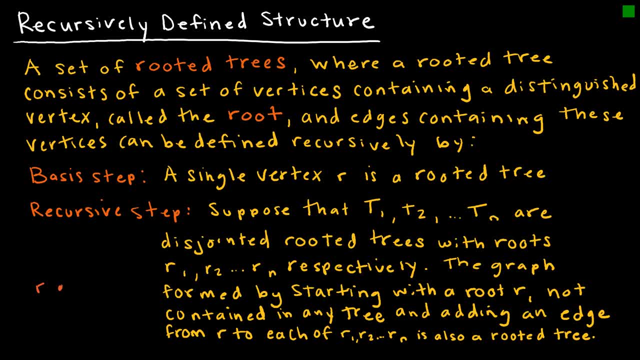 another, but they're all rooted trees with roots R1, R2, respectively. The graphed form, by starting with a root R that's not contained in a tree and adding an edge from R to each of those roots, is also a rooted tree. So let's say I have a rooted tree that looks like. 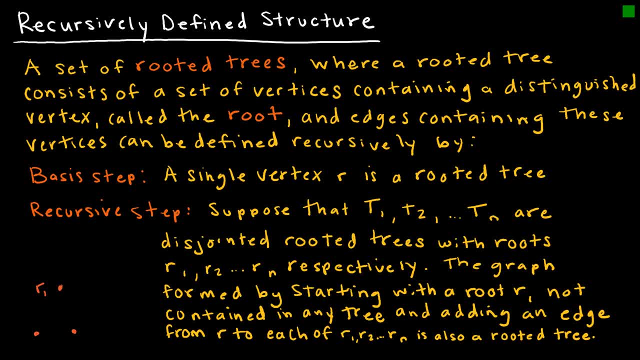 we'll call that R1, that looks like this: So that's my rooted tree. we'll call that tree 1.. And the recursive step says: hey, if I take a new root that is not contained in any other tree and I connect. 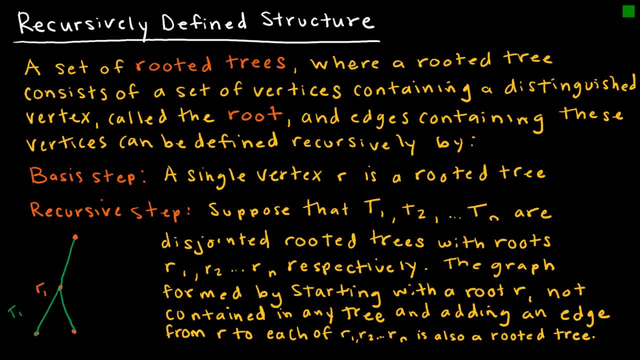 it to the other roots, then I have a rooted tree, So I connected it to tree 1.. Well, let's say I also had a tree 2.. Well, if tree 2 looks like this, which is disjoint, then the recursive step says: take that R and that. 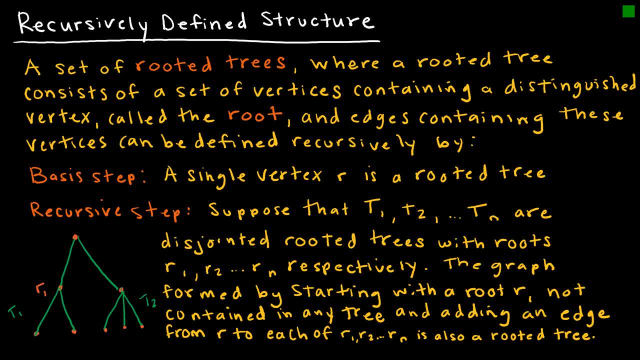 first- excuse me that- first root that's not part of a tree and connect it to those other trees, And now, all of a sudden, you still have a rooted tree. Obviously, that's a little bit larger, So let's take a look at what that would look like. 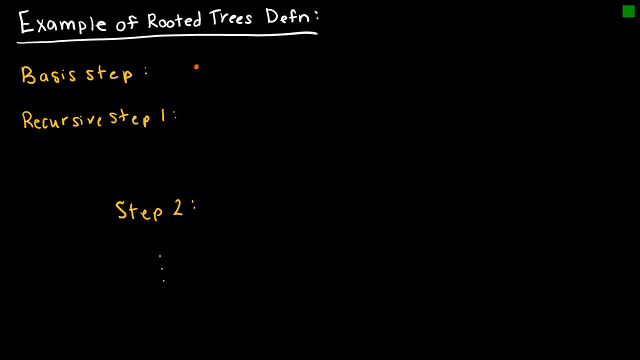 Using the recursive definition, the basis step again would just be one root. The recursive step says you can take that one root and add another root. You can take that one root and connect it to two others. You can take one root and connect it to three others And you get the idea I could. 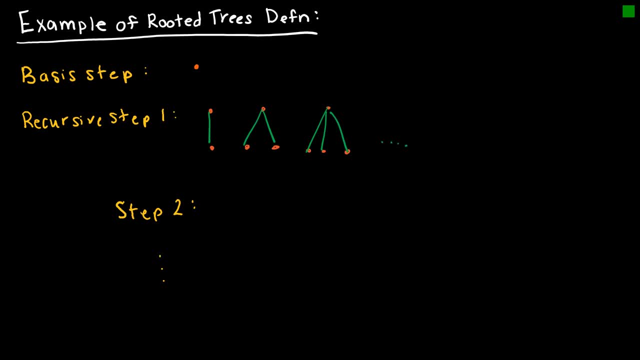 continue. If I then applied the definition again, the recursive step of the definition, again it's saying: take these structures that we came up with, which again go on forever, And now repeat that step again. So if I had my original, that looked just like this. that recursive algorithm says: hey, you can also just add one more if 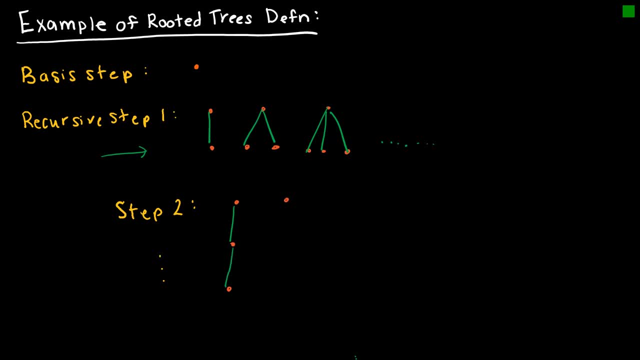 you want to, Or I could take my original that looks like this And I can take that one root and connect it to this And say: Okay, you can actually do two more off of that. Oops, that's the wrong color. You can do two more off of. 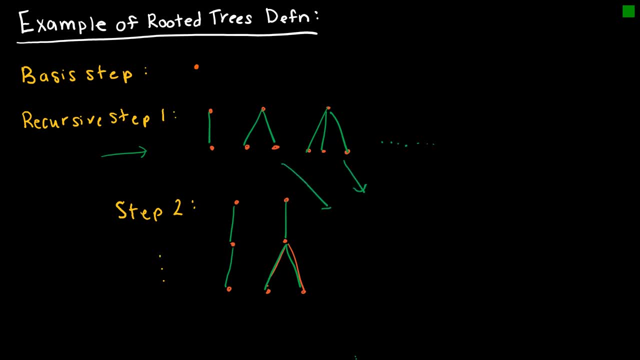 that Or I could have used this one and done the same thing, Or I could have used this one, Or I could have used one that I didn't even write down, And then, off of step three, I would be taking these structures and then adding: 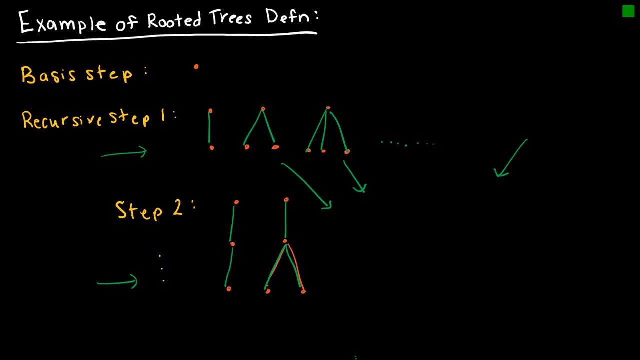 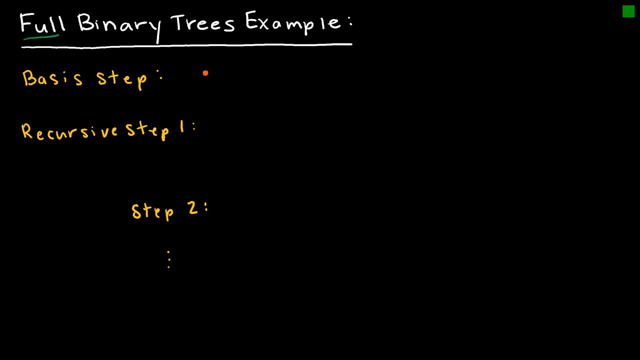 essentially another row, another height. I didn't write the definition for a binary tree. I did want to show you what a binary a full binary tree is. And a full binary tree again has the basis step of just a root. The recursive step one takes that root and connects it to two vertices Again, because this is a binary tree and binary.